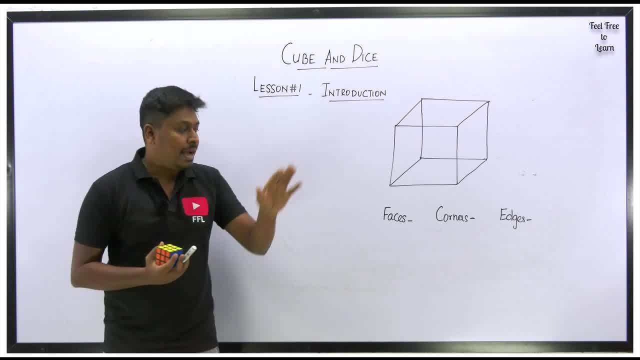 called dice. If you are preparing for a bank exam alone, only for the bank exams, kindly do not study this topic. Not even one question will be asked from this area. So if you are preparing only for the bank exams, you don't want to learn it. If you are preparing for other than bank exams, kindly 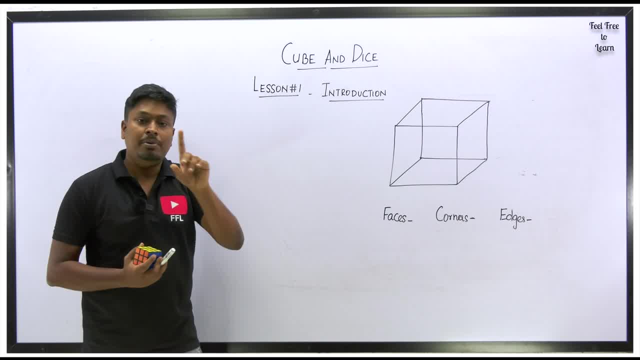 learn this topic. in every competitive exams you can able to see one question from the dice or else from the cube- Got it friends. So if you have to solve the question that is from a dice, so you have to know some of the questions from the dice. So if you have to solve the question from a dice, 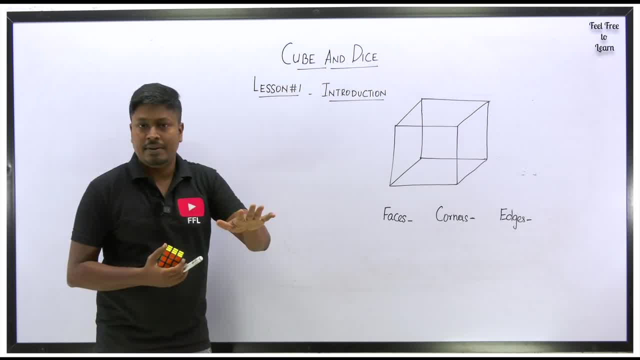 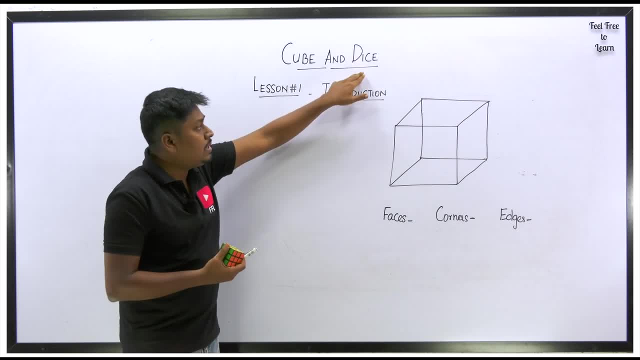 so you have to know some of the basic concept of cube. Some basic concept is enough. First week in this lesson number one, we are going to learn introduction about the topic called dice. But if you have to learn this dice, you have to know some basic about the cube. So that's the reason we are 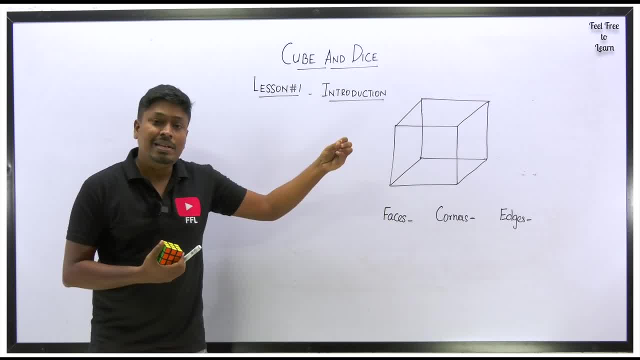 going to learn initially what is called as cube and what are all the important words in the topic cube, And then we can start learning the topic called dice. So first let me take the example here. You know how the cube looks like, So cube is called. what A square. 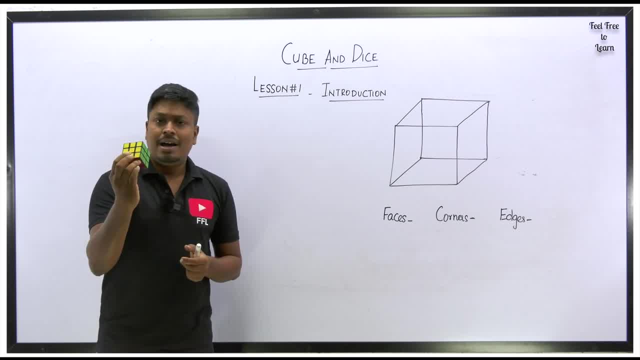 A square box. So you know cube looks like this structure. And why it is called as a square box? Because the length, breadth, height of all the sides will be same. So only then we call it as a cube. that is square box. If any one changes, then it is called as a cuboid, which is called as a rectangular. 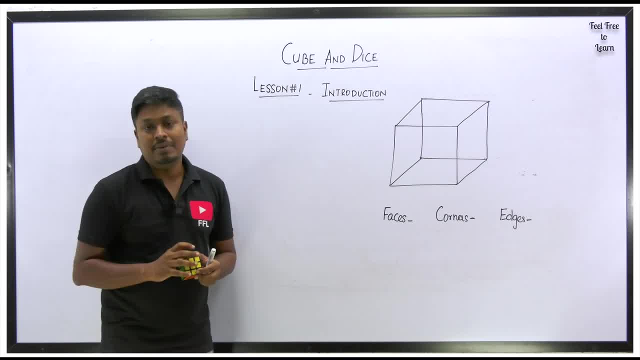 box. So here there are three important words. One is called as faces and second is called as corners and the edges. So you know, if you take this as a cube, right, it's a cube. So if you take this as a cube, 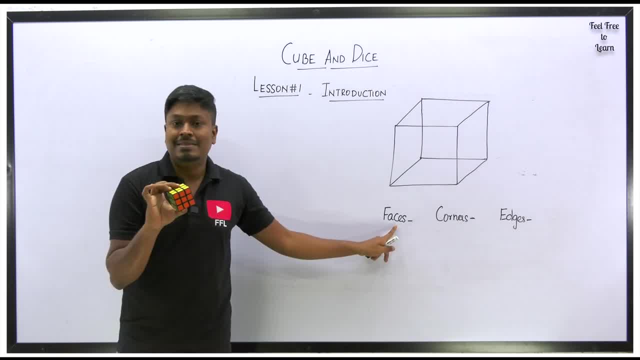 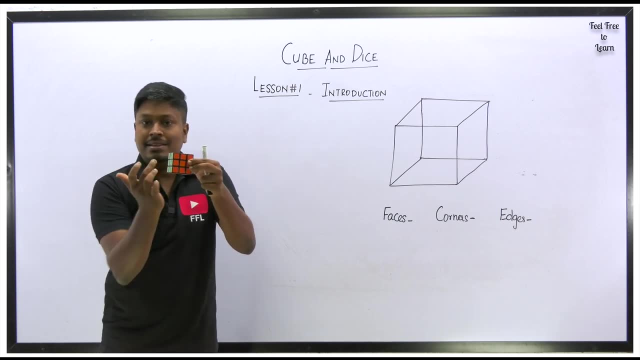 and what is called as faces. So faces is nothing but a surface area. For example, this will be one face, a top surface area, And this will be the bottom surface area, which they usually call it as a bottom face. So top face, bottom face and the front facing, back facing and the right. 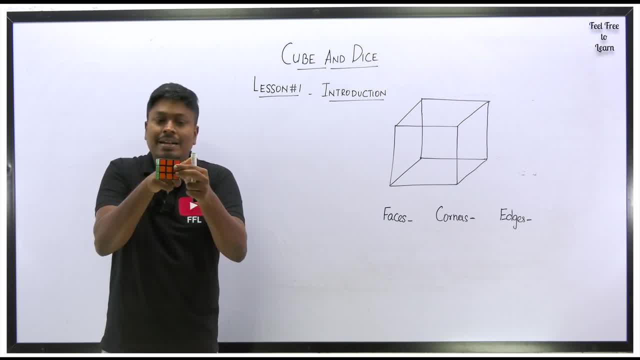 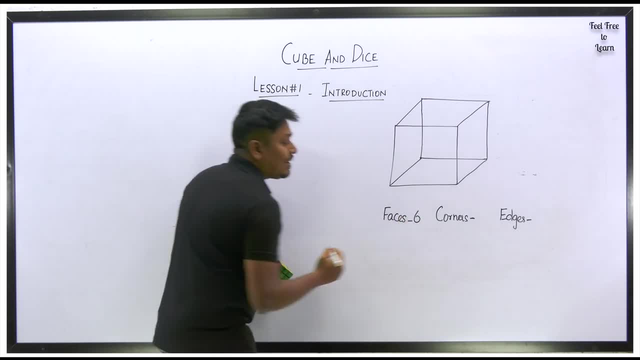 facing. For me it is right, but for you it is left right. So right facing and the left facing. So totally, how many faces are there? Six faces are there, So we can say that for a cube there are six faces, Got it. So next is the corners. So corners is nothing but this point. 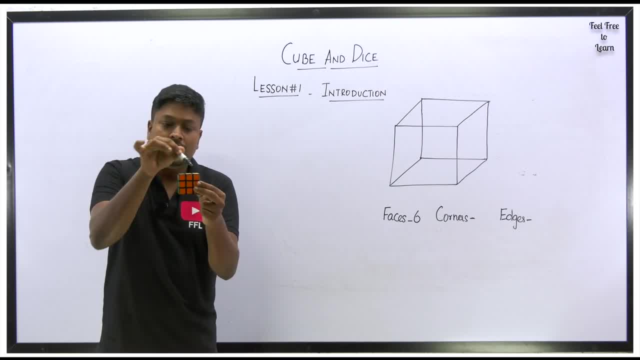 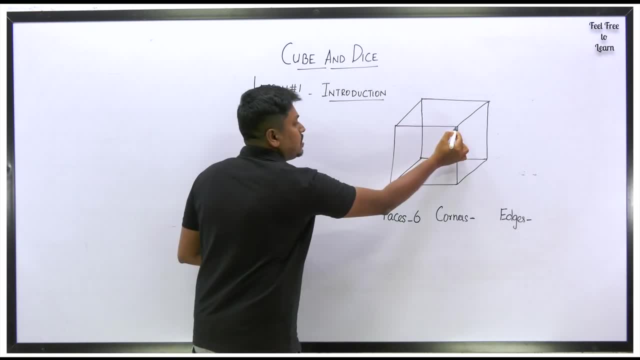 is called as a corner. If you take a cube this will be one corner, two corners, three, four, five. So each point this is called as one corner, understood. So one, two, three, four, five, six. 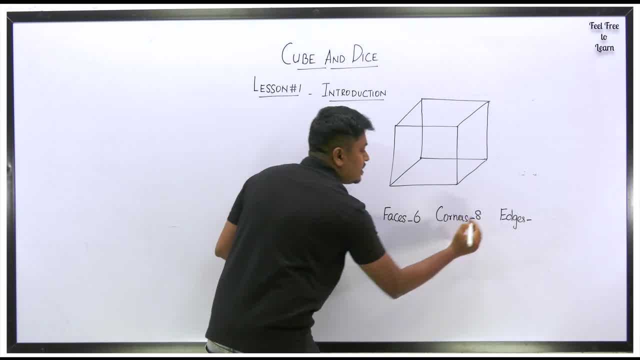 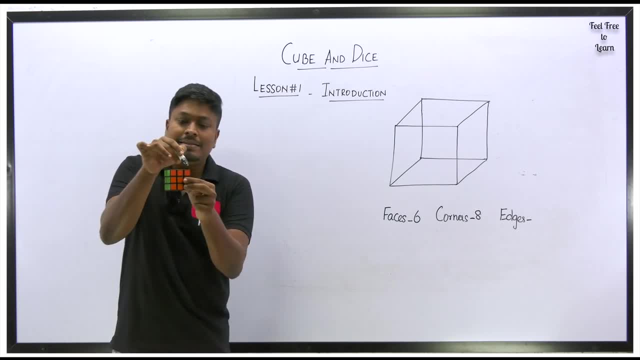 seven and eight. So totally how many corners are there? Eight corners are there And the last is called as the edges. So what is called as edges? You can see when you take this cube. this is called as an edges or no. This is one surface. 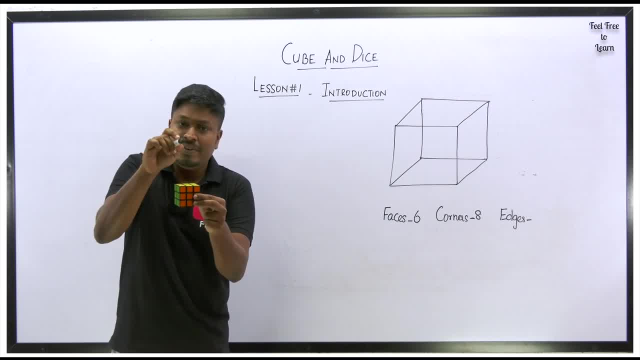 area. So this will be the top surface area. In this top surface area we can say this complete area is called as edge, edge of the surface. When you take this surface right, when you take this surface, the edge of the surface will be this, this and this and this. So this is called as. 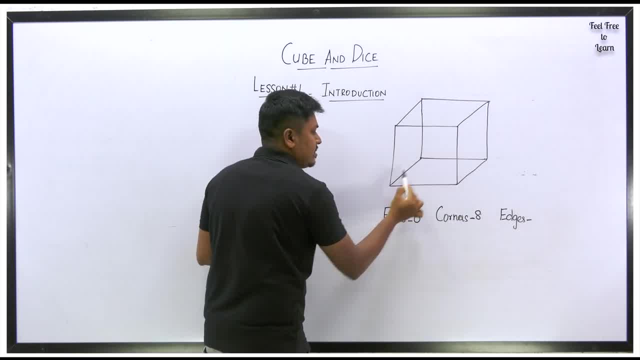 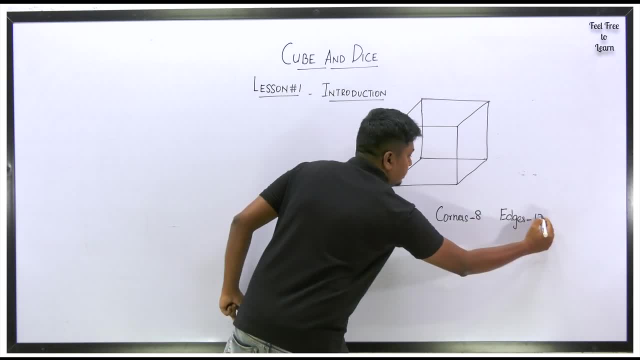 an edges, Got it or not, So this line is called as an edges. Or else simply keep that in mind: all the lines is called as an edges, So we can say, totally there are 12 edges, So that's it, So totally. we have three important words in the topic cube. One is a faces and 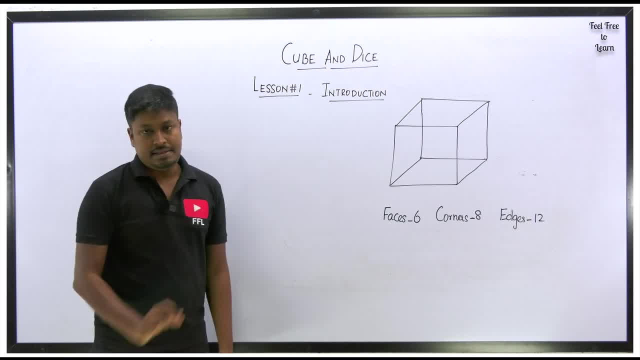 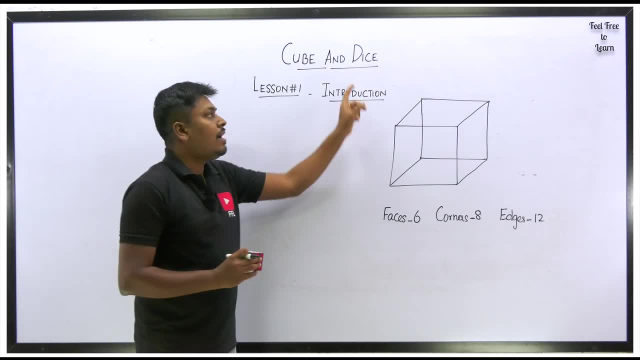 second is the corners and the third is called as the edges. I hope you understood the concept right. So this is more than enough. right, By knowing these three stuff, you can able to solve 100% of the question from the topic called dice. So now entering into the concept called dice. 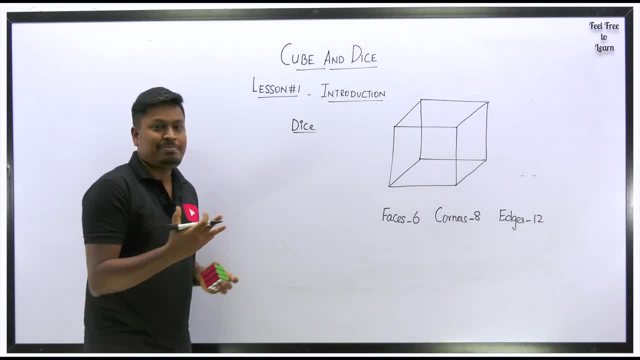 So, friends, everyone have seen the dice In the childhood times. we usually play that Ludo, Snake and Ladder Only by using this dice right. But when you come to this quantitative aptitude dice, there are two type of dice. One is called as a standard dice Standard and the second is called as a general. 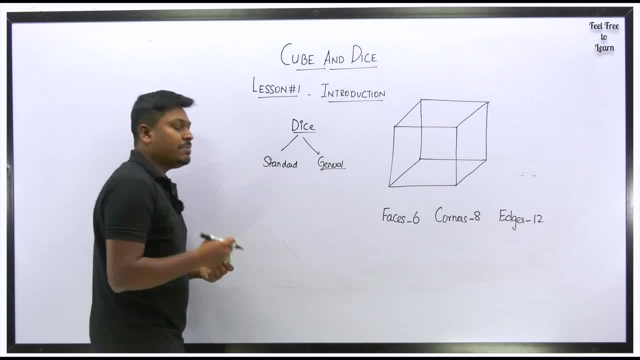 dice. So, friends, listen here this same general dice. some students will call it as a non-standard dice. So totally. the dice has two types. One is a standard dice and the second is the general dice, or else a non-standard. 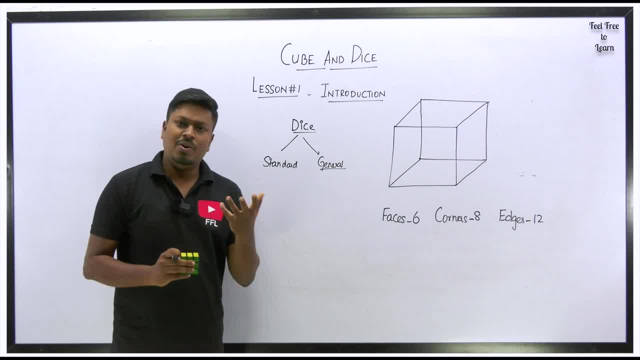 So first entering into the concept called dice, You know how the dice looks like. So in the childhood times we know that there will be a one dot at the top, So we just call it as number one, two dot, three dot, four dot, etc. In the childhood times what we used to play that Ludo and Snake. 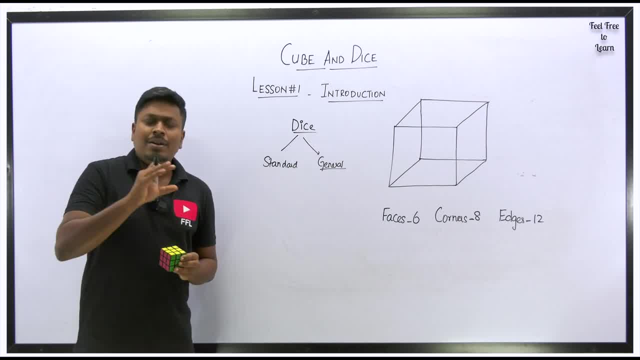 and Ladder. it is a standard dice. So what is the difference between standard dice and a general dice or a non-standard dice is just listen here. some of most important thing- some right, some of opposite faces- is seven. That is most important. Just listen carefully. 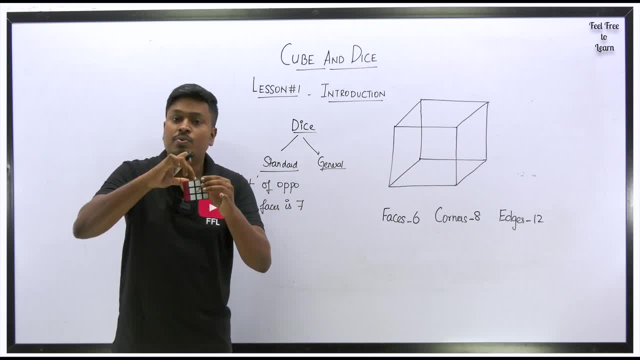 For example- let me keep this as a dice right- If the top is one, there is one dot right. If top is one, then the opposite face. we know that it is an upper face, top face, So the bottom face will. 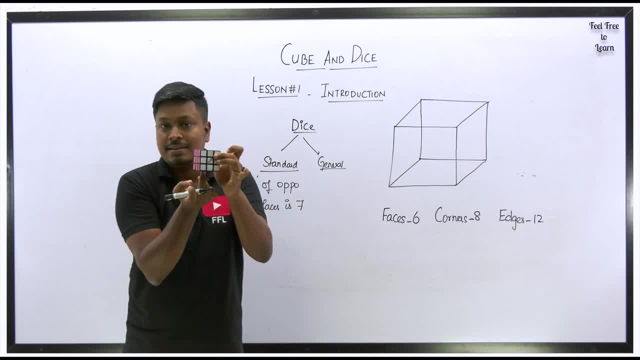 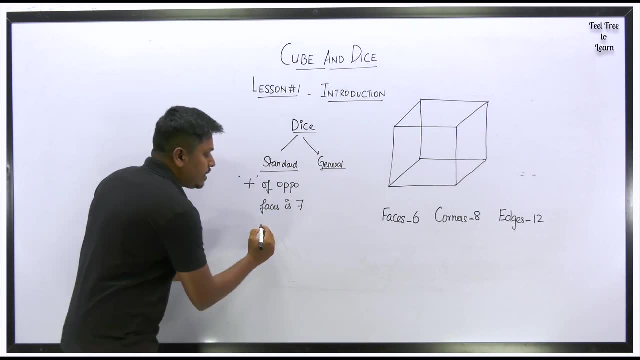 be six. If it is one, the bottom face will be six. Only then we can say that if you add the top face to the bottom face, six, the resultant will be seven. Always remember that sum of opposite faces should be seven, right? If the top face is two. right, For example, if this is two, right then. 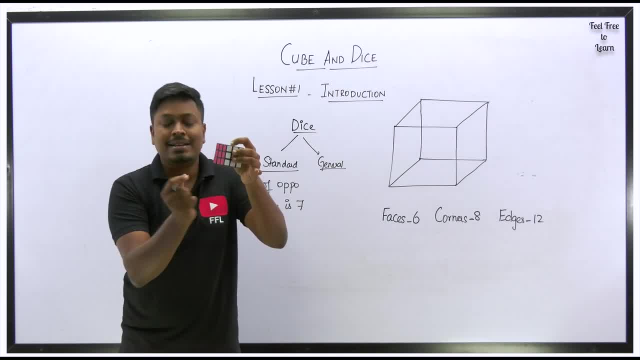 what will be the bottom face? The bottom face will be five. Only then we can say that five plus two will be seven. In case if this face is four, for example, I am saying this face if this face is four. if they are asking what is the opposite face number, if this is four, then this will be three. 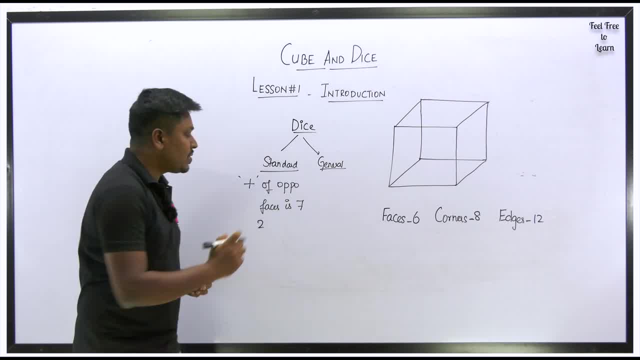 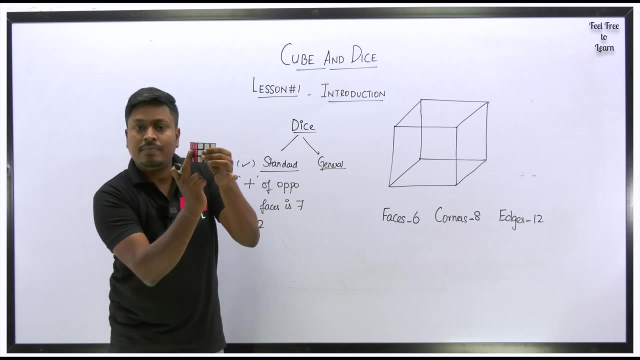 So only then we can say that four plus three will be seven, which is called as a standard dice. So never forget it. Sum of right, Sum of sum, is nothing but addition. Addition of opposite faces will be seven. Got it. If this is one, this will be six. If this side is four, this will be three. 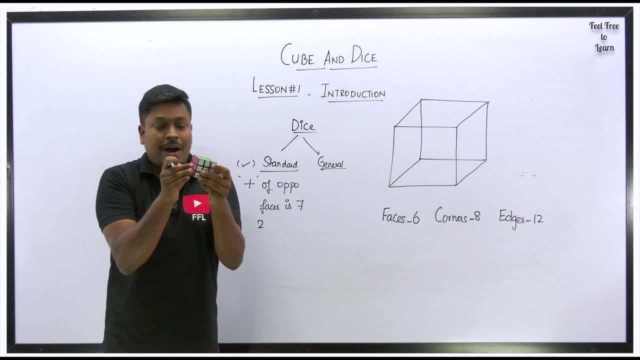 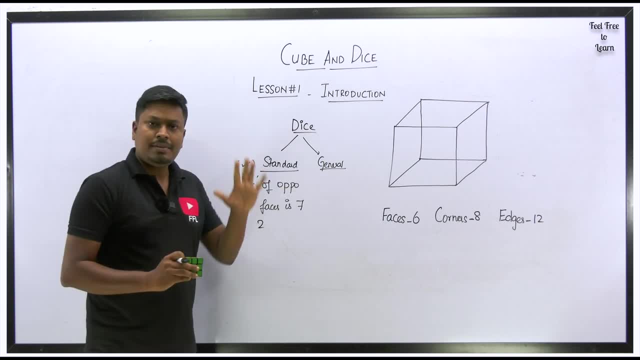 If this side is five, then the opposite side will be two. So addition of all the opposite faces, the total will be seven. Then it is called as a standard dice. Usually play the games only by using a standard dice, right? So now a general dice or a non-standard? 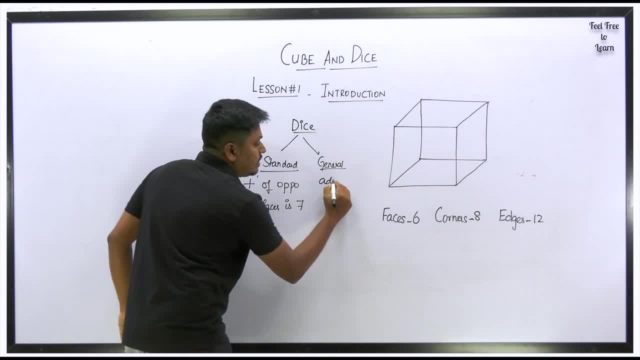 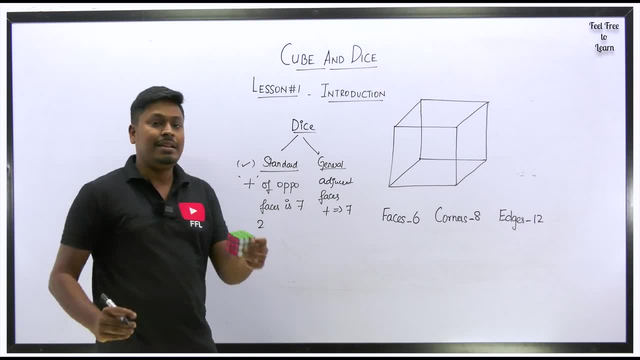 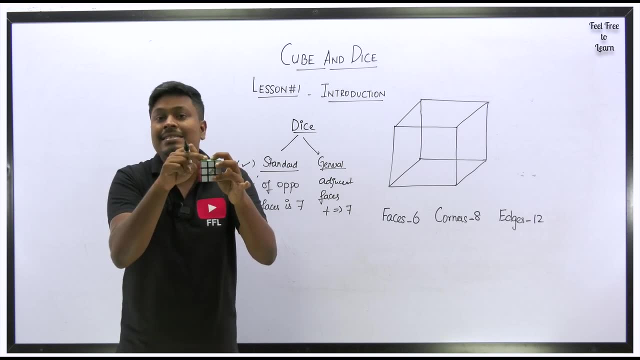 dice. Listen here. Here the adjacent, adjacent faces sum is equals to seven, Got it? Adjacent face is nothing. but for example, if this face, top face, is six, example, I am saying, if top face is six, then the adjacent, adjacent is nothing but a neighbor. A neighbor face will be one Only. 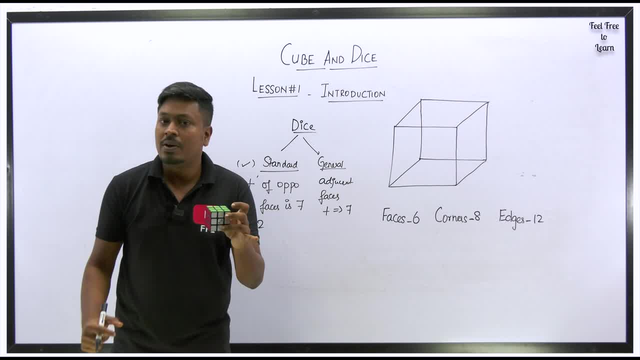 then when you add six and one, you will get a number. So if this is one, this will be three. The resultant will be seven. Got it or not? In case, if this face is five, then the adjacent side, either this side or this side, will be two. Only then we can say: five plus two will be seven. 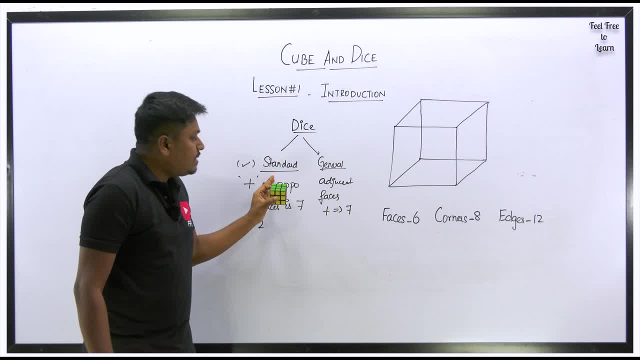 Got it, friends. So the difference between a standard dice and a general dice, What is the major difference? When you take a standard dice, the opposite side sum will be seven. When you take a general dice, the nearby faces total will be seven. That is called as. 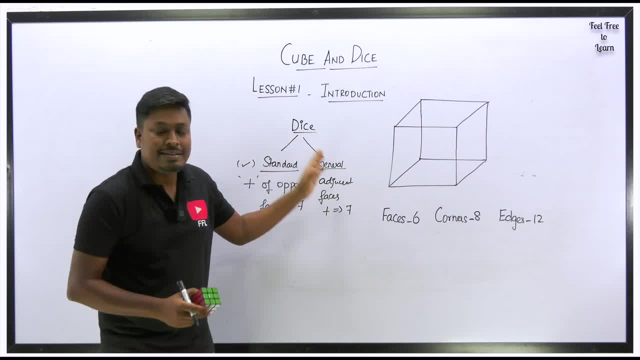 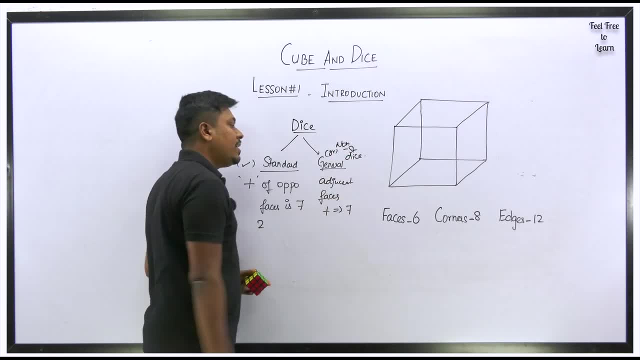 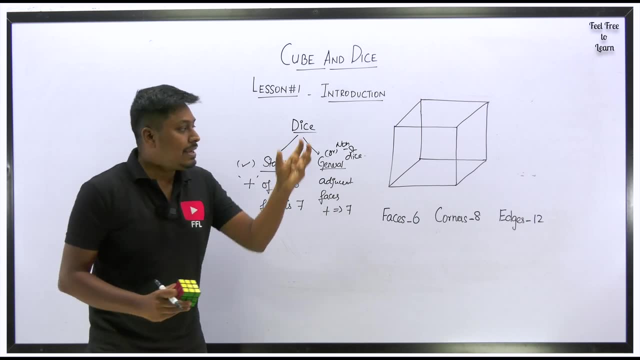 the difference between a standard dice and a general dice, Or else this same general dice are also called as non-standard dice. So got it, friends. So before solving every question on the topic dice, first you guys have to decide: the given image is a standard dice or a general dice. 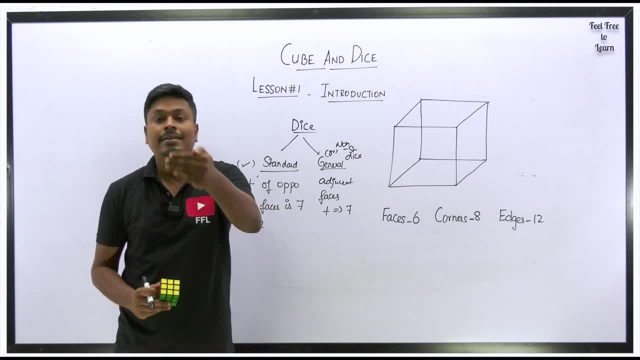 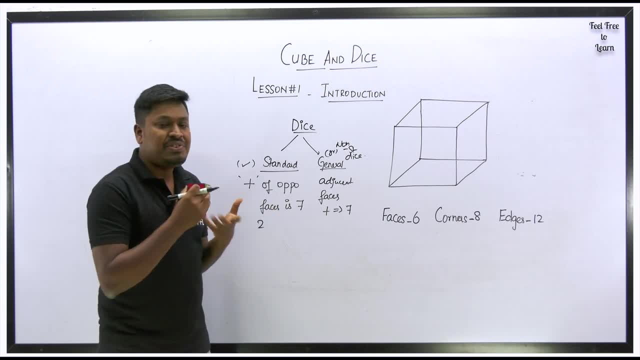 That is important. So, after knowing which dice it is, and then start solving the question. So only then you will feel easy. And second most important thing is you have to know the answer to the question us. we have many shortcuts, many techniques and many different methods to solve a question dice. 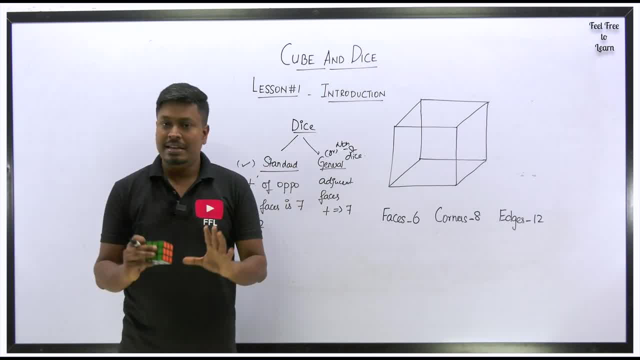 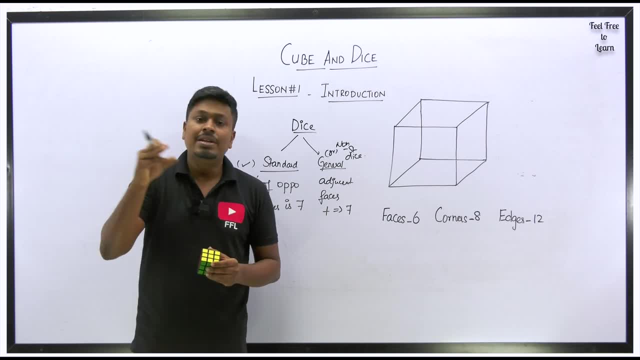 but try to learn any one or two method. that is enough. don't learn all the shortcuts. right for solving one question there will be five to six shortcuts, so don't learn all the shortcuts. try to learn out of five, one or two which might be helping you to solve all the hundred percentage. 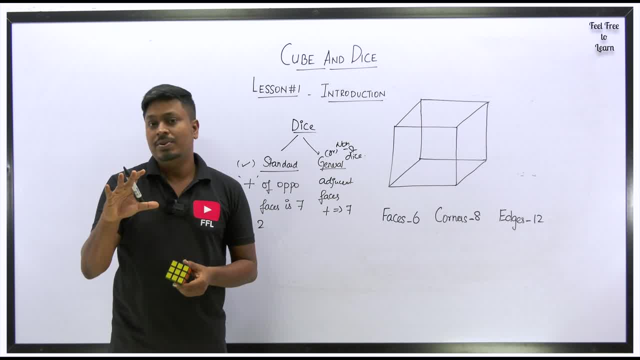 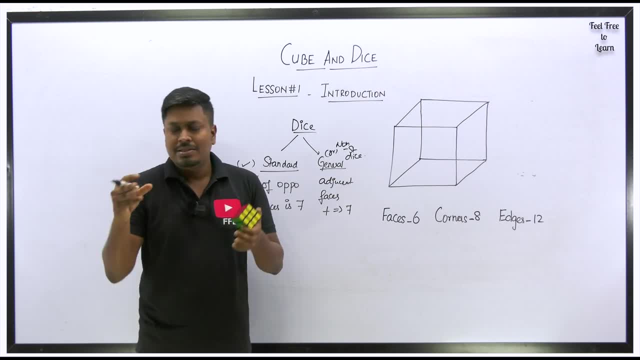 of the questions in the topic dice. so don't learn all the five shortcuts. if you learn all the five shortcuts, you will get confused while solving some difficult question. so that's the reason i'm saying: out of five, so try to pick one or two and try to be strong on those shortcuts. right. so now? 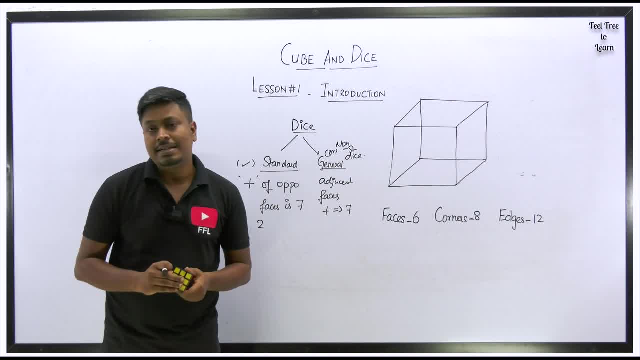 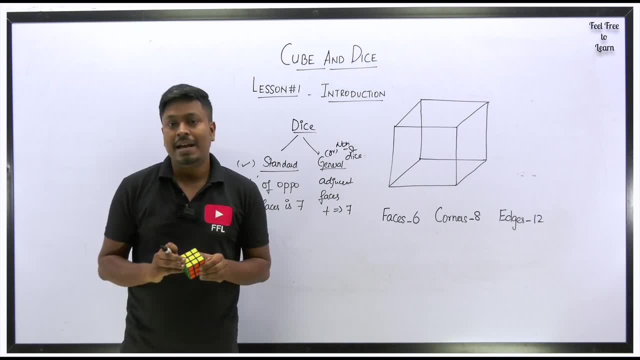 entering into some basic example of dice. we can see that. so before seeing that example of dice question, just listen here how the questions and your exams will be asked. what are all the shapes you can able to see? usually the exam question will be like: they will show you what is the top. 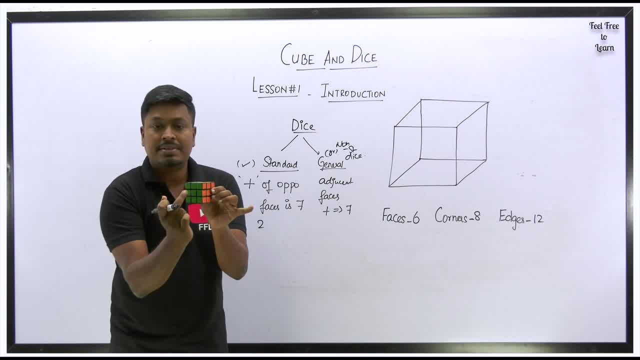 face number. got it. this face number and this face number, so only these three faces will be visible in your paper exam papers. got it? they usually show a image like this. so here you can able to see. you can able to see the top face as well, as you can able to see this side- both the sides- but you can't able to. 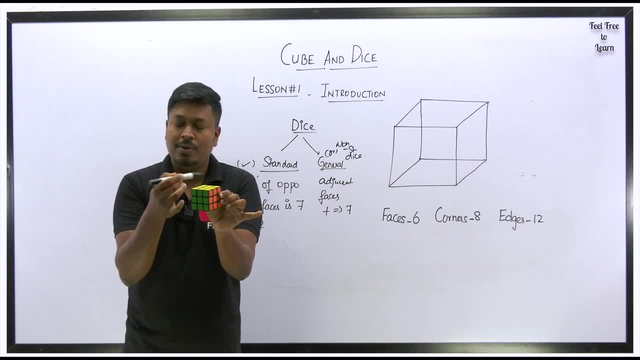 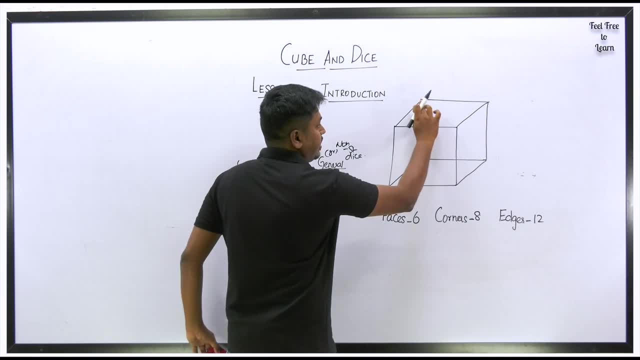 see the bottom face and this and this got it or not, right. always remember that in the exams they usually show you only three faces. what else i can draw this image like this? just see here: they will show you the top right, so they will show you this top face and they will show you the front face and also the 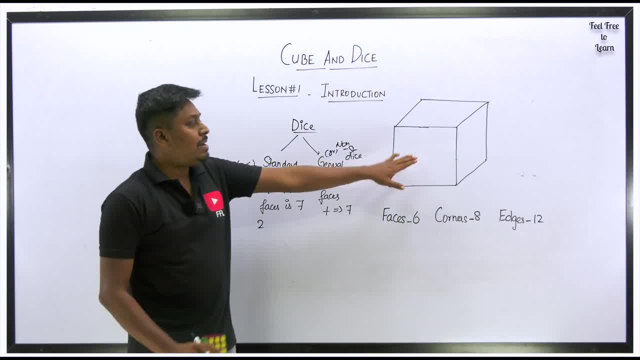 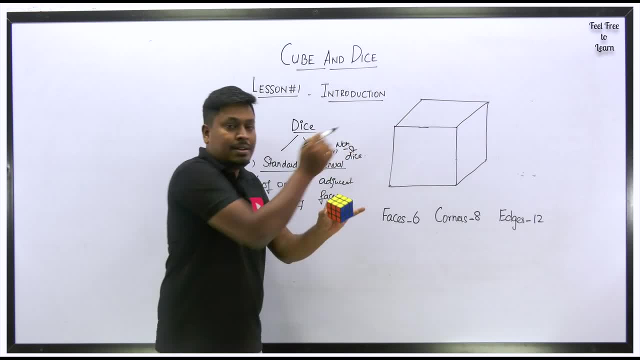 side face got it? usually in the exams they will give a image like this which determines the cube is exactly like this, got it or not? so you can able to see the top face. this will be the top face right and these two side faces are visible. so now let me enter into some of the example questions. 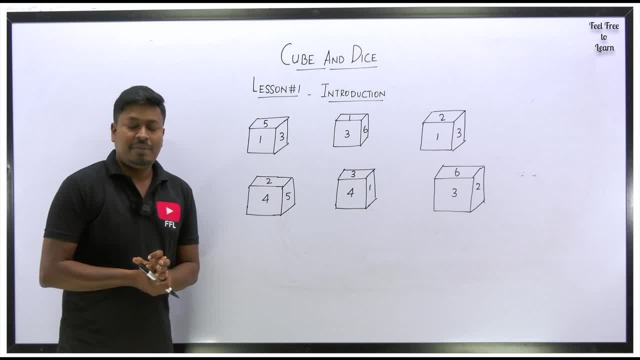 so, friends, here i have taken six example question. so our target is to find whether the given dice is a standard dice or a general dice. you know what is the difference, right? so first let me move on to this example question one. just see, here you can able to see three faces. so this will. 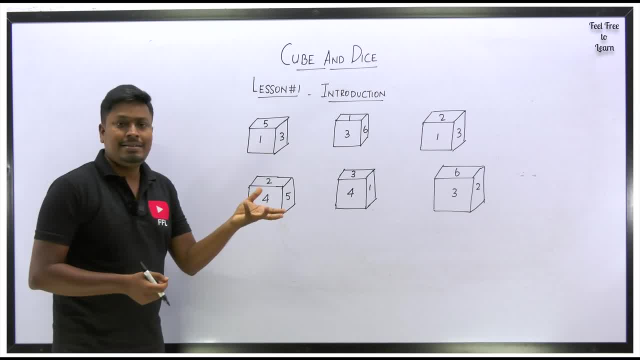 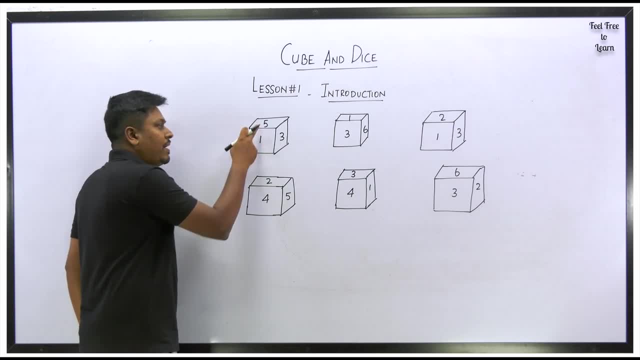 be one face, second face and the third face. usually in the exams they will always give you three faces. so in this three faces they have denoted by a number. the first face, the top face, is five and here the number is one and here the number is three. whether the given dice is a general dice. 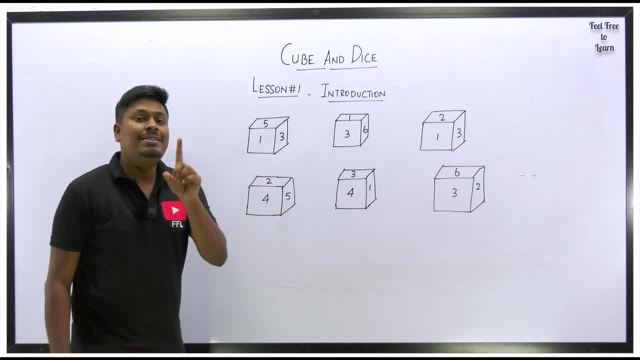 or a standard dice. just check what i have told you. if it is a standard dice, if it is a standard dice, the opposite faces. while you add opposite faces, the resultant will be seven, what is called as general dice. if it is a general dice, if you add the adjacent side, the total will be seven. just see, five plus three is what eight. 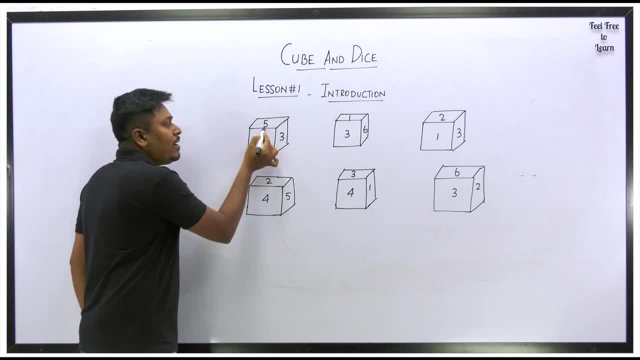 three plus one is what four? so when you add all these adjacent faces then it is not a total, is not seven. so definitely we can say that the given dice will be a standard dice. so friends got it or not understood what i did. so what i did is i have added: 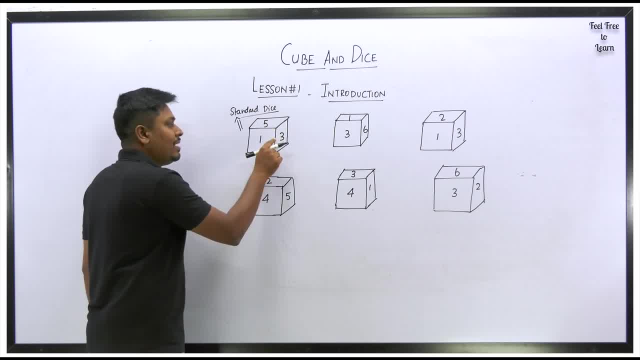 all these faces. five plus three is eight, so not seven. three plus one is four, not seven. five plus one is six, not seven. so while adding all these adjacent faces, i am not getting a total seven. if i am not getting a total seven, then it will be a standard dice in case if i get a total of seven. 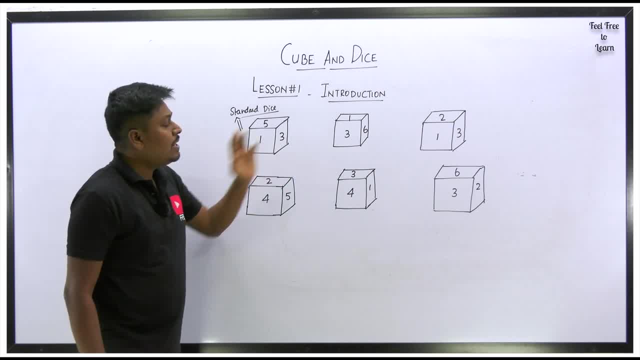 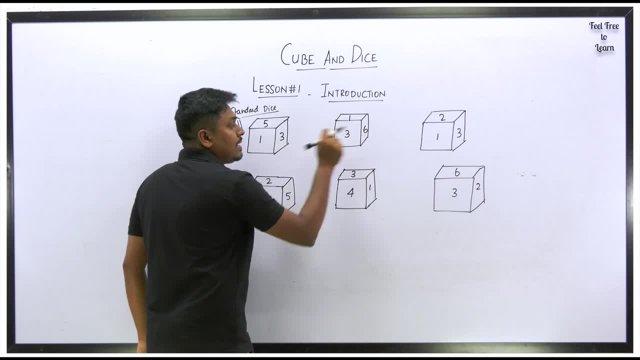 then it is called as a general dice. so let me move on to the second example. just see, here we have three faces: the face, the top face, is one and the side face is three and this side face is six. so what you need to do, you have to check. 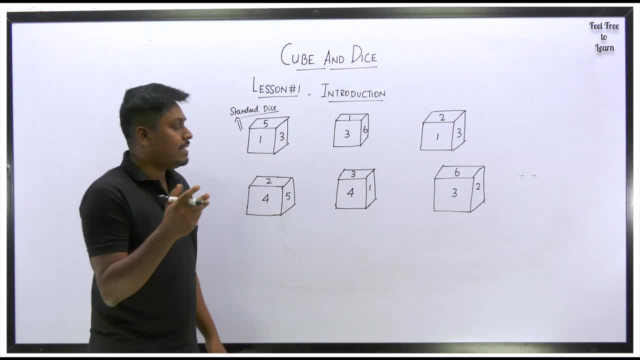 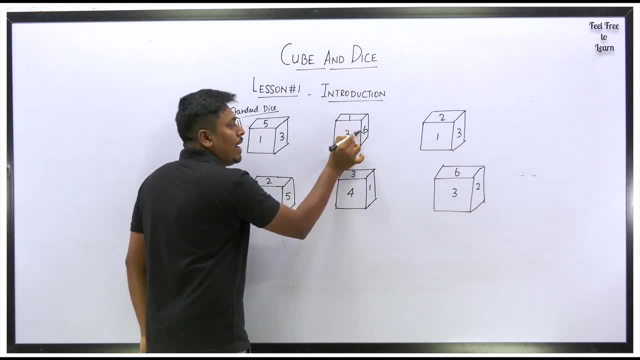 this and you have to say the dice is a standard dice or a general dice. just see here, when you add the adjacent side. so three plus one is four. one plus six is what. just see while adding the adjacent faces. six plus one is what- seven. so while adding the adjacent face, i am getting a number seven. 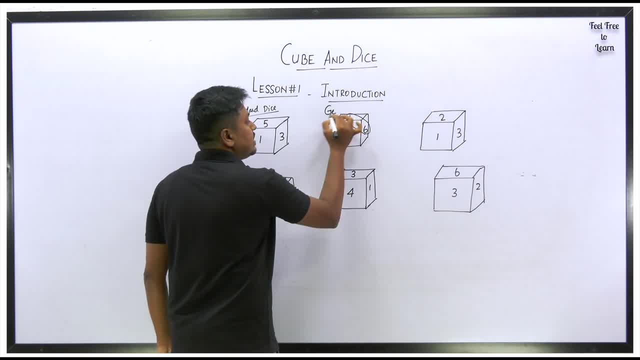 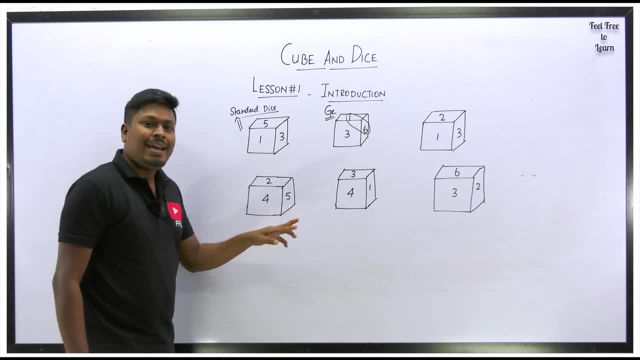 then it is called as a general dice. so friends got it or not? so similarly, let me move on to this example. so two, four and five. so add any two adjacent faces. if i add five plus four is nine, no, four plus two is six, no. when you add five plus two again, we are getting a total. what total is? 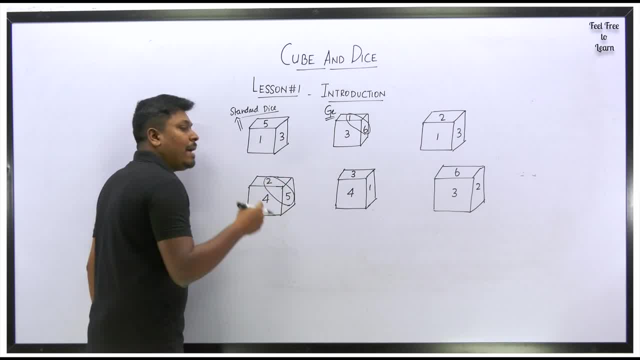 seven. so while adding this adjacent faces, i am getting a total of seven. if i add the adjacent faces and i am getting a total of seven, then it is called as a general dice. so, friends, got it or not? then it is called as what? non-standard dice, or else it is called as a general dice, so friends. 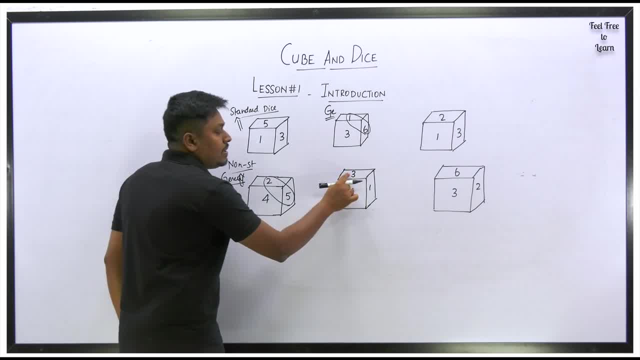 got it. so another example: so three, one and four, just add the adjacent faces. if i add three plus one, resultant will be four. no, so four plus one is five. no, four plus three is what again, when you add four and three, these two adjacent faces, i am getting seven. so while adding the adjacent faces, 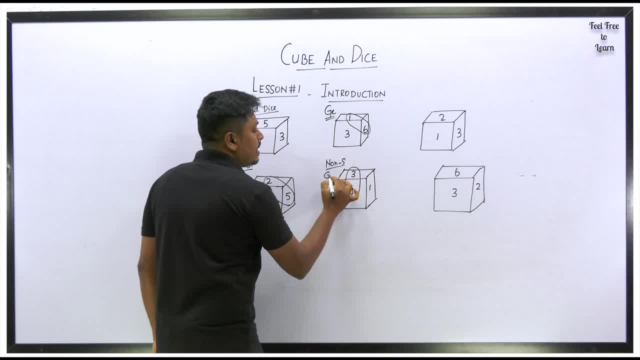 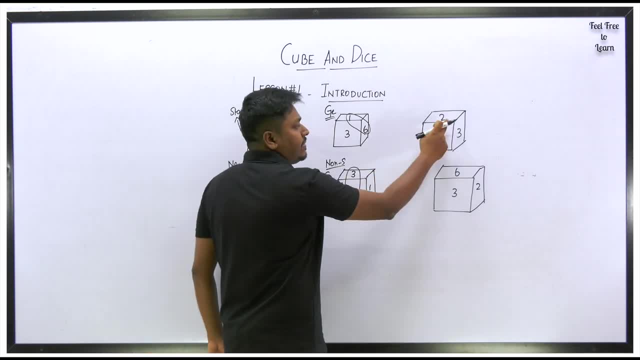 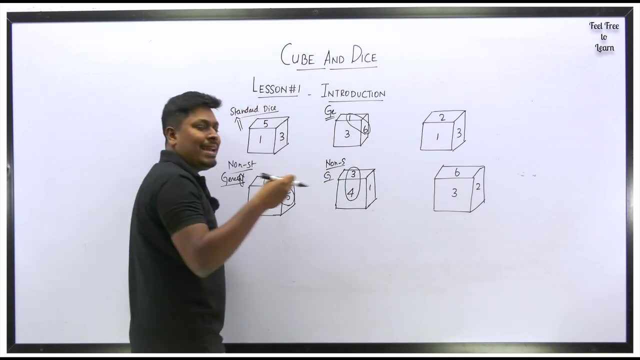 so definitely it is a non-standard dice or else it is a general dice. got it, friends. so next one, two and three. so just just add and check with adjacent faces. so two plus three is five, not seven. three plus one is four, two plus one is three. so while adding all any of the two adjacent faces, i am not. 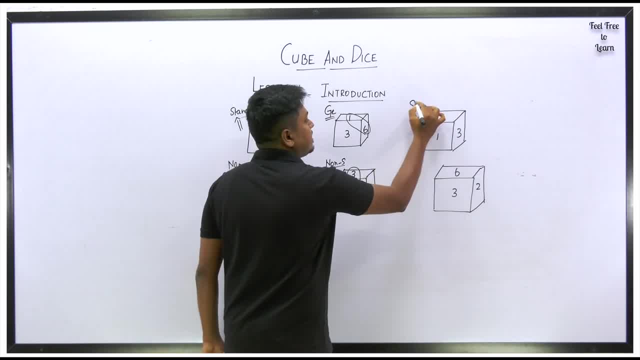 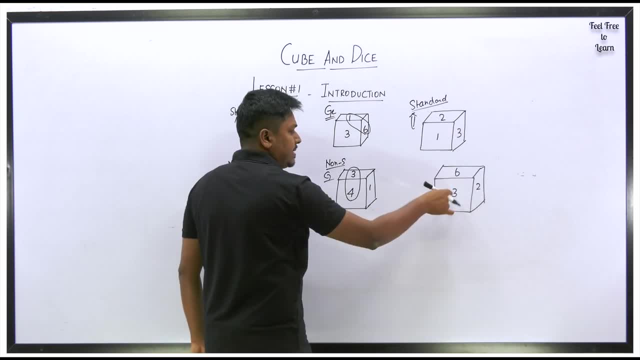 getting a total seven, then it is called as: what a standard dice? standard dice: got it or not, friends? so, similarly, if you add six plus two is eight. no, six plus two is eight. no, six plus two is eight. six plus three is nine. three plus two is five. so while adding any two faces, i am not getting seven. 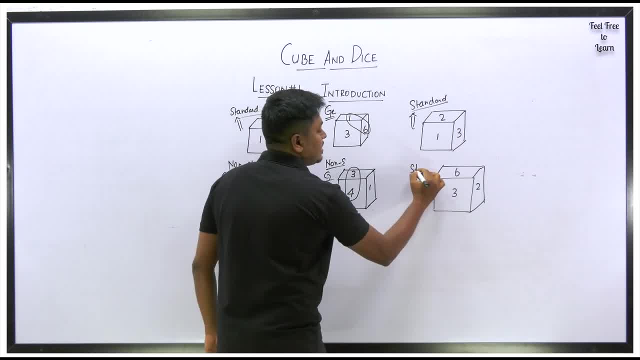 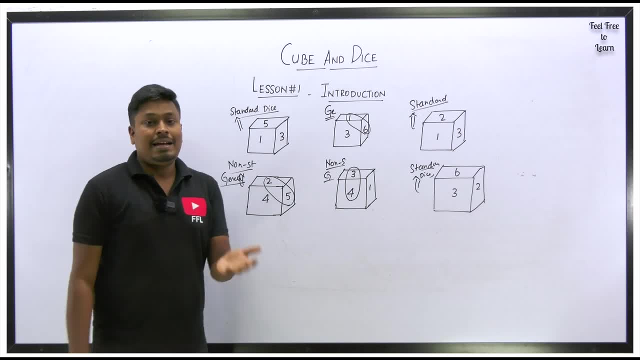 if i am not getting seven, then it is called as a standard dice. that's it, friends. i hope now you understood what is the difference between a standard dice and a general dice. got it so usually every time while seeing the questions in your exam. first you have to decide whether the 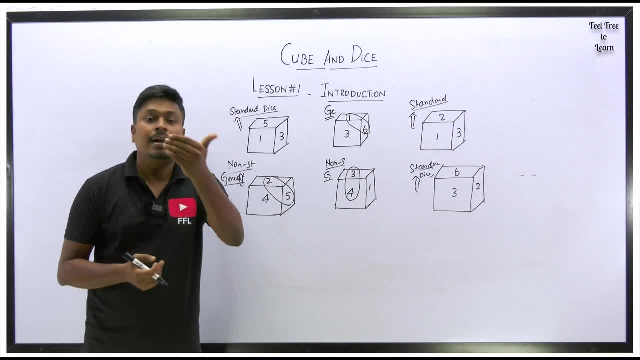 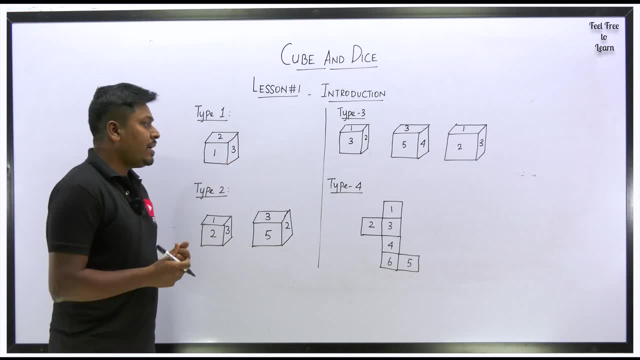 given dice is a standard dice or a general dice, and then start solving the question by using the standard dice, so entering into the last session of this introduction video. so here we are going to learn totally. there are four types of questions they can ask from the topic dice, right, so? and 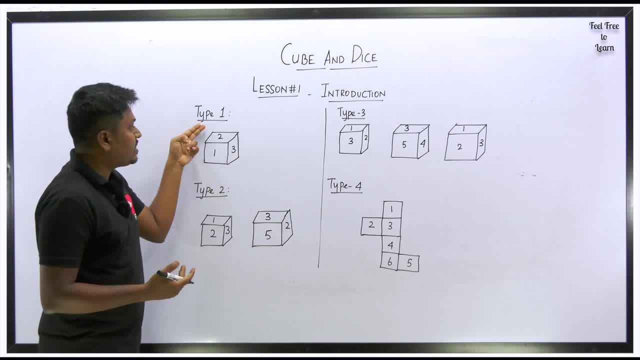 then from the upcoming videos, that is lesson number two. we are going to solve some question from type one, then lesson three, lesson four, lesson five, etc. so before that you have to know what is the different type of question they can ask from the topic dice. so type number one: type number one. 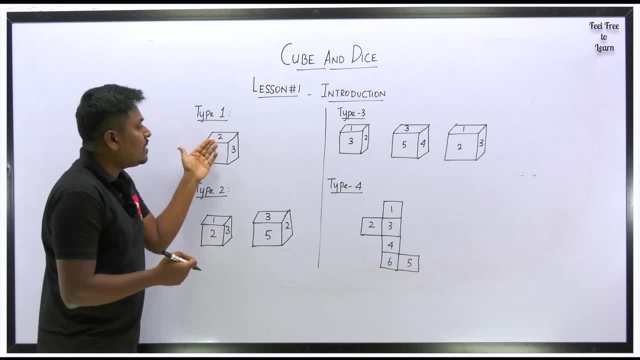 usually they will give you only one dice, so, based on that, they will ask us a question, for example: what is the opposite face of three? they can ask a question like this by giving one sort of images, and they will ask you that: what is the opposite face of three? right, so you have to. 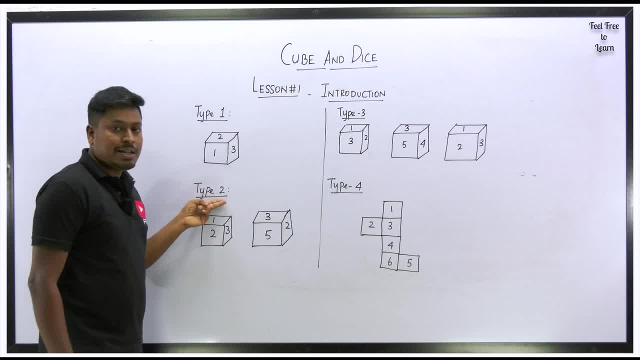 think and you have to write down the number. so, similarly, type number two is nothing, but they will give you two dice and based on the two dice, they will ask you a question: for example, what is the opposite of number three? got it. so, similarly, type number three will be more than two, it can not only. 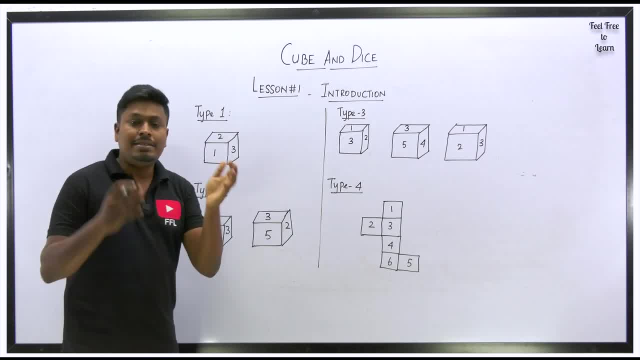 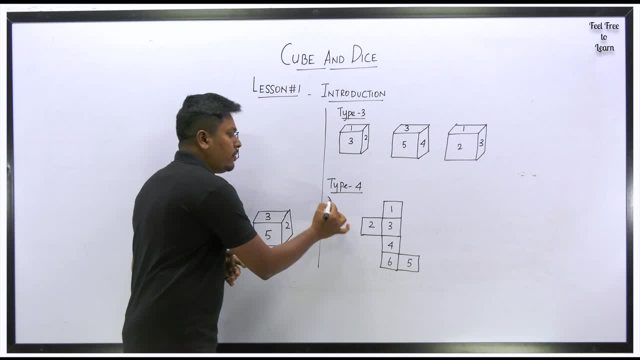 be three or four, etc. they can give you four or five dice based upon the five days. they will ask you some sort of question and we have to solve it, which is called as type number three. so type number four is a different type and most important type also. so here you can able to see they will.